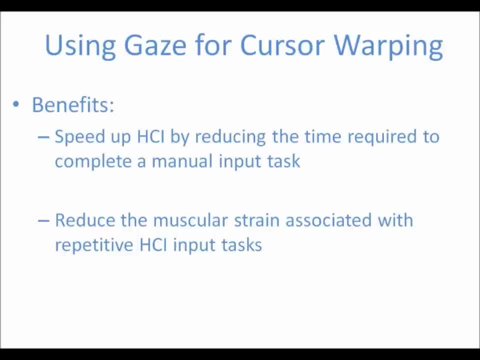 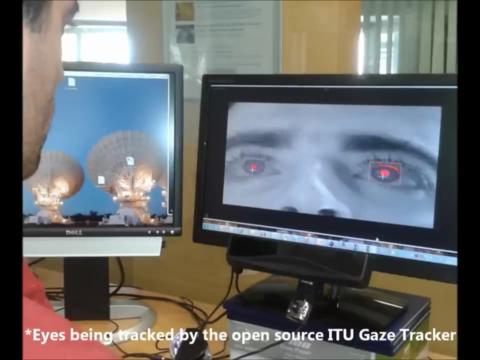 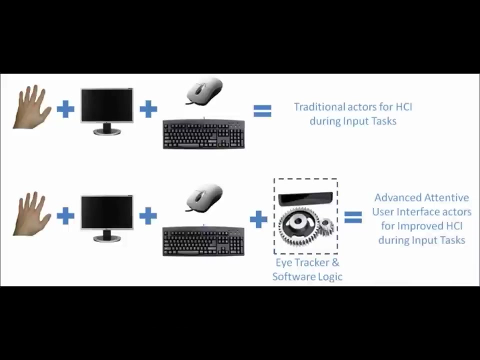 Specifically, we show how a large part of the manual movement required to reposition a mouse or keyboard cursor can be eliminated by warping the cursor towards the user point of regard on the screen, as estimated using gaze estimation algorithms. The method combines both manual input from the user to indicate intent and final fine-grained positioning of the cursor and an attentive user interface. 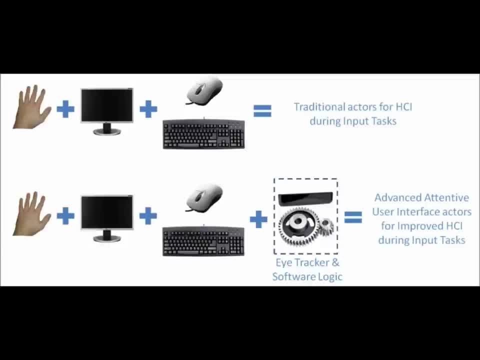 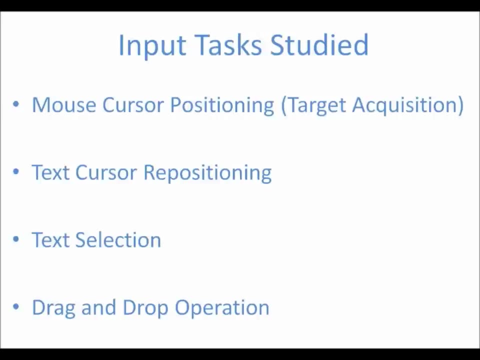 that adapts the cursor position dynamically according to the user, manual input and gaze position on the screen. We have studied four common tasks carried out during human-computer interaction: Target acquisition, text cursor repositioning to text selection and a drag-and-drop operation. 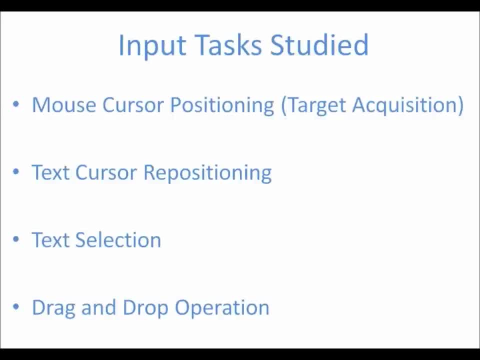 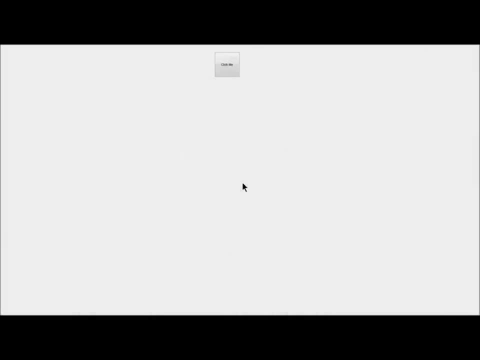 Let's look now how cursor warping can speed up and reduce the muscular strain associated to common input tasks- Input tasks during human-computer interaction. For the mouse cursor warping experiment, the subject is first required to click at a random target on the screen for 10 trials. 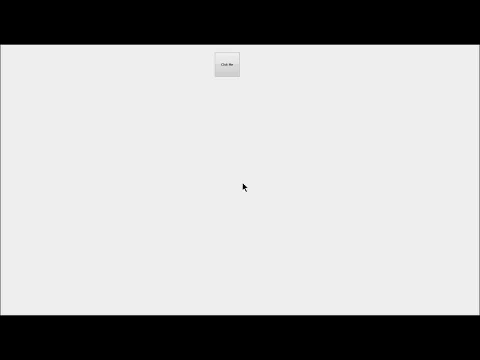 For each trial, both the target and the mouse cursor appear at a random position on the screen, So the subject simply has to click at the random target for 10 trials. Mouse cursor warping consists of making the mouse cursor jump to the area of the screen where the user's gaze is estimated to be placed. 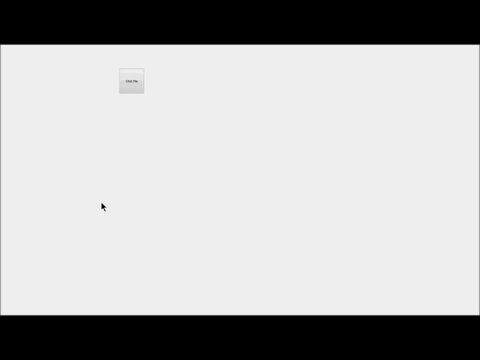 whenever a slight mouse movement is detected and proven that the mouse has been quiet or stationary for a few seconds. So, for example, we see that the mouse cursor in this screen is situated at the center of the screen If the user looks at the click-me target and then moves the mouse slightly. 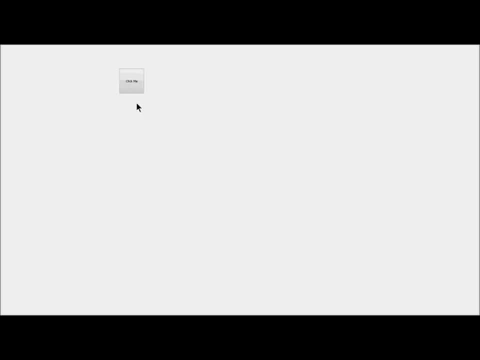 the mouse will jump to the gaze estimation area and then the user just completes the clicking on the target by manually moving the mouse. To better visualize what is happening in this experiment, we have generated a red dot that moves around the screen and which indicates the user's gaze coordinates as estimated by the gaze tracking algorithms. 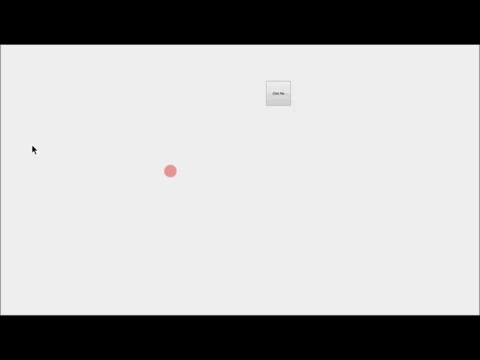 So at this moment in time, I'm looking at the center of the screen and the mouse cursor warping consists on the fact that the mouse cursor is in this area of the screen and whenever I look at the target that I have to click, if I move the mouse slightly, the mouse cursor jumps to wherever I am looking at. 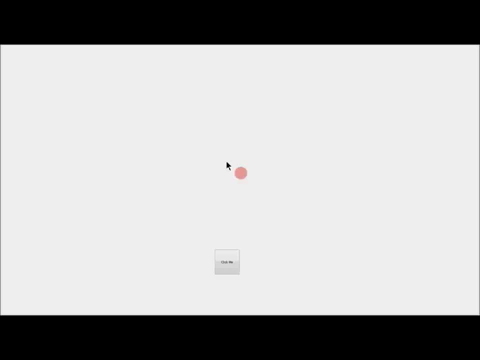 and then I complete the selection by clicking on the target To minimize overshooting of the mouse cursor. when placed over the target according to the gaze estimation area, the cursor position can be offset towards the incoming path of the manual mouse-actuation vector. 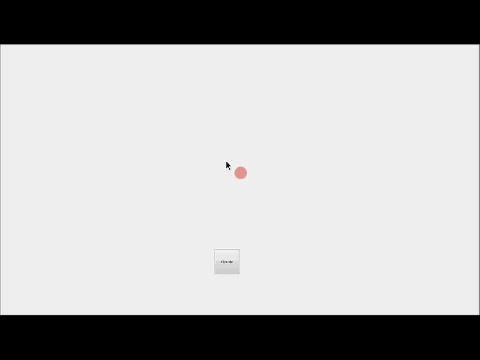 And this sensation mechanism can be put in place by which, instead of placing the cursor at the center of the gaze estimation area, the cursor position can be offset towards the incoming path of the manual mouse-actuation vector. This technique increases the time required to perform target acquisition. 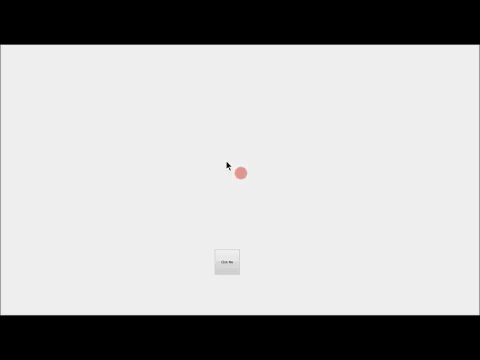 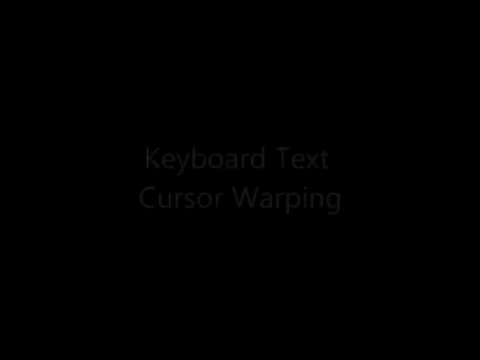 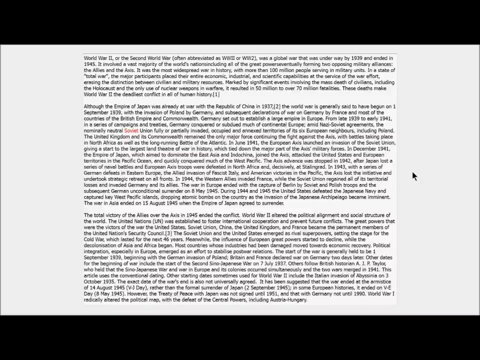 but makes the cursor appear in motion towards the target after the warping occurs, which some users find convenient. Some of the most impressive results of using the warping concept and gaze tracking technology to speed up human-computer interaction were obtained in the text cursor warping experiments. 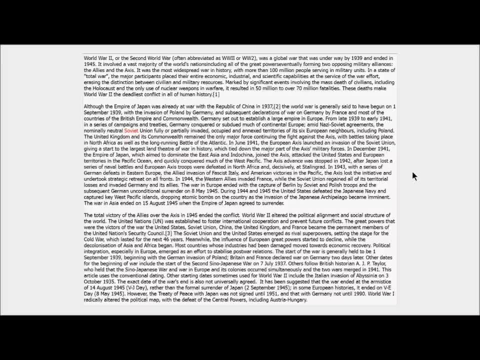 In these experiments, the users or the subjects were requested to place a keyboard text cursor within the boundaries of a word highlighted in red. In the control experiment, the word appeared at a random position for 10 trials and the text cursor was also placed at a random position. 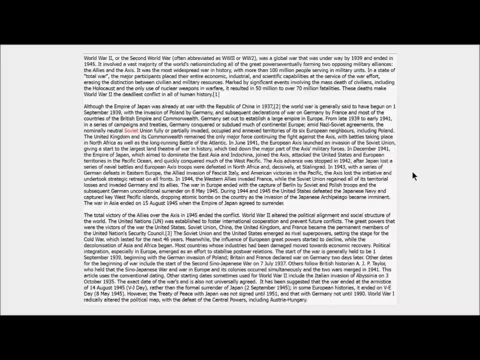 Subjects were requested to position the text keyboard cursor within the red word, both first using the keyboard and in another experiment, using the mouse. So just by using the direction keys or any combination of control keys plus direction keys, you can position the text cursor in a random position. 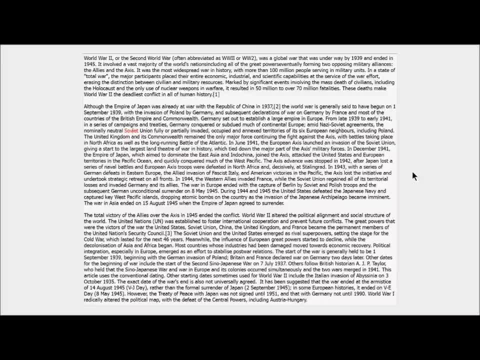 In this case the text cursor was carried to within the highlighted word and at this time the timing watch was stopped. Then the subjects moved to the next trial by pressing F1 and there's a new word highlighted in red and the text cursor has been placed at a random position. so the user just has. 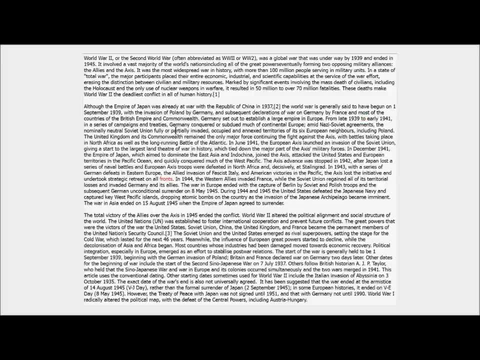 to bring the mouse cursor to within the word And do that for 10 trials. Using text cursor warping consists on moving the keyboard text cursor to the area of the screen where the user is gazing at, which, for this task, would be around the word highlighted. 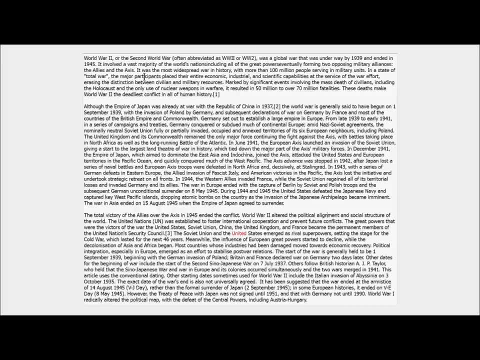 in red and whenever a direction key is detected, to be pressed, making the text cursor jump towards the highlighted word. So, for example, here we see that the text cursor is in the word alignment. the target to which we have to bring the text cursor is here. 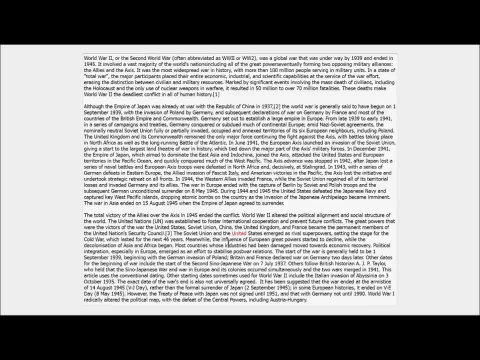 And if we look at the text cursor, we can see that the text cursor is in the word alignment, so we can click on it and press any direction key. the keyboard cursor jumps to the vicinity of the word and then we complete the selection manually using the keyboard key. 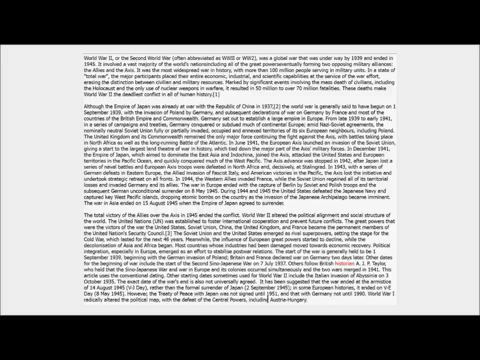 We do it for another interaction. the task here is the text cursor and we jump the text cursor towards the target word just by pressing only a few times the direction keys. Here is the text cursor, here is the highlighted word. We look at it, we press a few times the direction keys and the cursor jumps to the vicinity of the word. 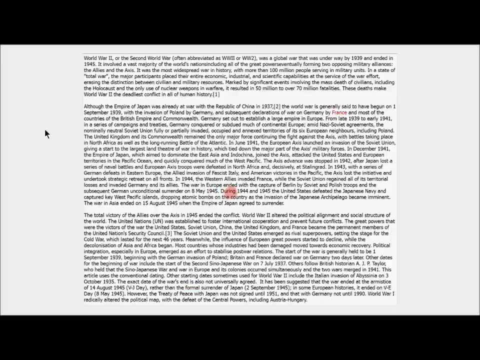 Again, using the visualization of the gaze estimation area helps a lot to illustrate the concept. So at this moment my gaze is looking at the vicinity of where the text cursor is, and if I look at the target word and I click a direction key, the text cursor is within the vicinity of the word, and then I complete the task manually. 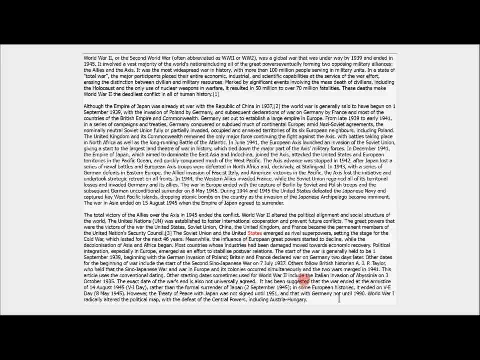 Let's do it for a few times. Here is the random position in which the text cursor is. The cursor has been placed, here is the target word and I move towards it in just three keystrokes. Again, here is the text cursor, the target word, and I quickly move to it. 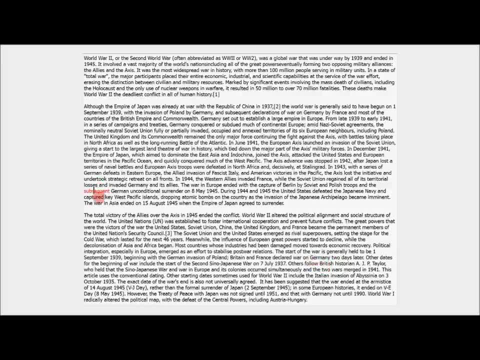 Let's do it for a few times Again. here is the text cursor, the target word, and I quickly move to it in just three keystrokes. For the text selection experiment, two words appear highlighted on the screen: one in blue, one in red. 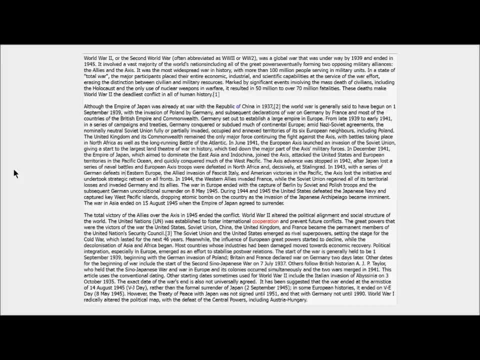 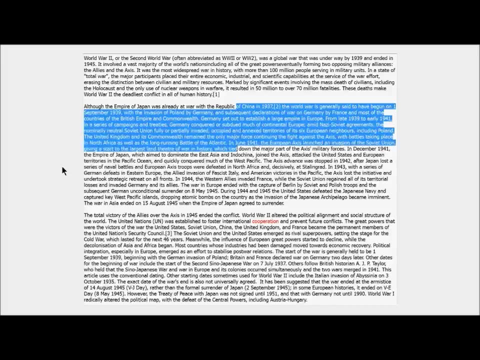 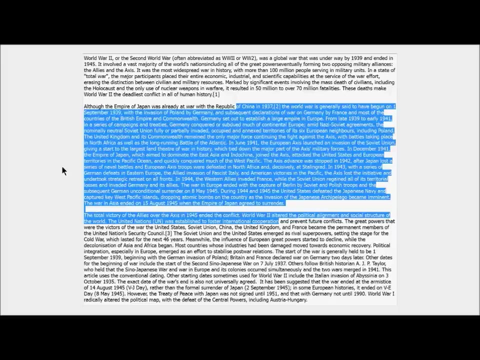 The idea is to select all the text between both words and starting always the selection from the blue word. So the idea is like the cursor again appears in a random position and we bring the cursor towards the blue war and we initiate the selection and complete it all the way to the red war and then we press F5 to stop the time watch and to finalize the counting of the keystrokes required to complete the task. 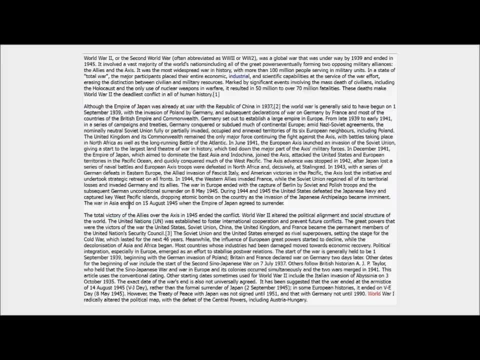 So the task- using cursor warping to complete this task- consists on first looking at the blue war, then initiating the selection and looking at the red war, and both times the cursor should jump to the vicinity of where the person is looking at. So we look at the blue war and we press any direction key and the cursor jumps to the vicinity of the war, and then we initiate the selection by pressing F5 to stop the time watch and to finalize the counting of the keystrokes required to complete the task. So the task using cursor warping to complete this task consists on first looking at the blue war and then we press F5 to stop the time watch and to finalize the counting of the keystrokes required to complete the task. So the task using cursor warping to complete this task consists on first looking at the blue war and then we press F5 to stop the time watch and to finalize the counting of the keystrokes required to complete the task. So the task using cursor warping to complete this task consists on first looking at the blue war and then we press F5 to stop the time watch and to finalize the counting of the keystrokes required to complete the task. So the task using cursor warping to complete this task consists on first looking at the blue war and then we press F5 to stop the time watch and to finalize the counting of the keystrokes required to complete the task. 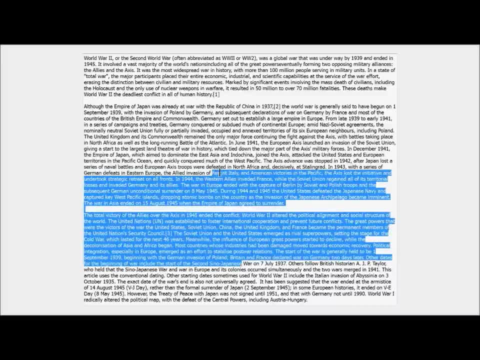 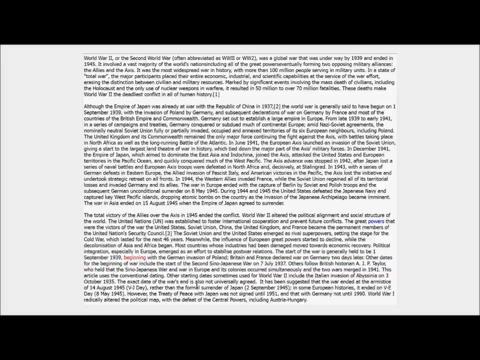 And then the selection should jump to the vicinity, where we only have to do a few keystrokes to complete the selection. Once again, the mouse cursor is at a random position here and we look at the blue wall and press any direction key, The text cursor jumps to the vicinity of the wall. 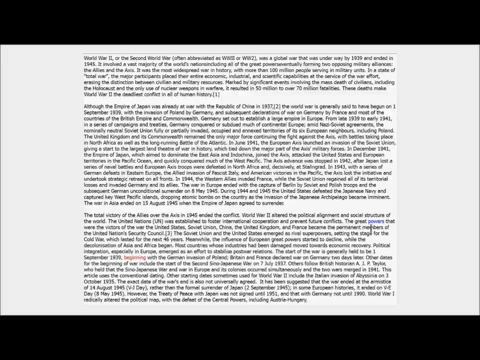 We initiate the selection by pressing and holding the shift key. We look at the red wall and the selection is almost completed. Once again, showing the visualization of the user's gaze helps a lot to illustrate the concept. So, for example, I'm looking now at the random position where the text cursor is located. 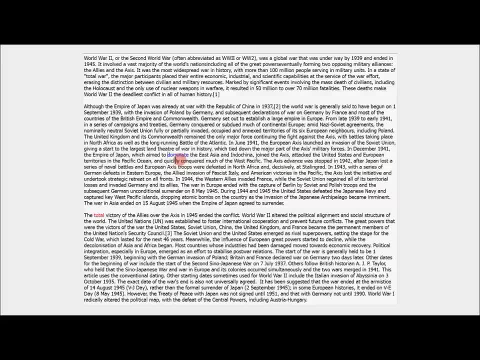 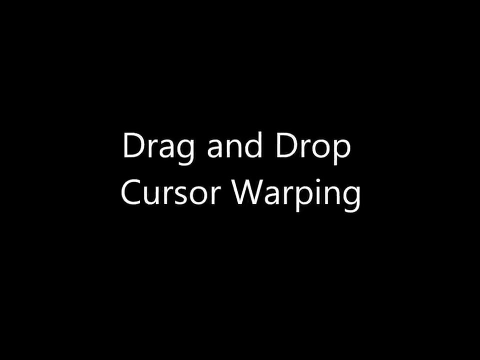 I look at the blue wall, The text cursor jumps to the vicinity of the wall And then I look at the red wall and I press and hold shift, move, Press any direction key and the selection is almost completed For the drag and drop. 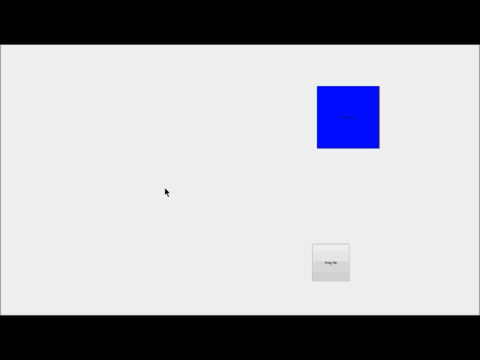 For the drag and drop experiment. the idea is to drag the grey target into the blue target using a traditional drag and drop operation. For each interaction or trial, the mouse cursor and both targets appear in random positions. The process for performing a drag and drop operation using cursor warping is a bit more elaborate and probably it has a step learning curve. 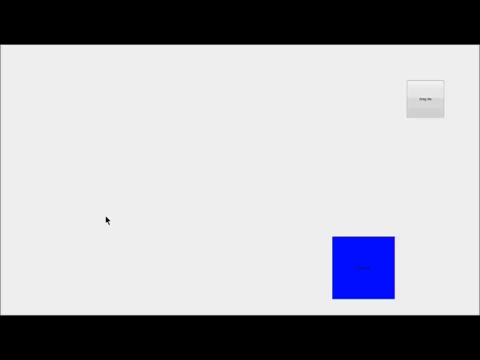 The idea is to look at the first target, the grey target, and then move the mouse slightly. By doing this, the cursor jumps to the vicinity of the button. Then we press and hold the left button of the mouse and look at the blue target and move the mouse slightly again towards the blue target. 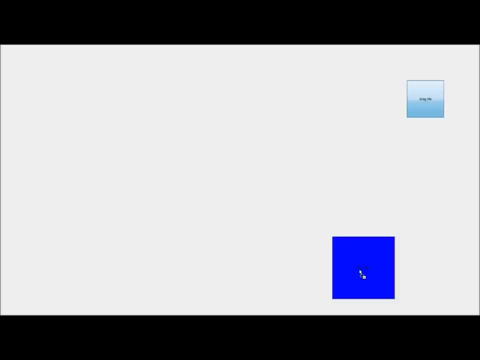 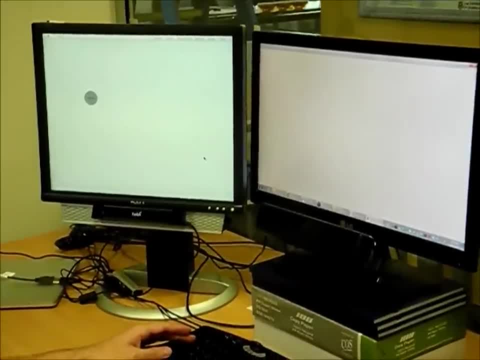 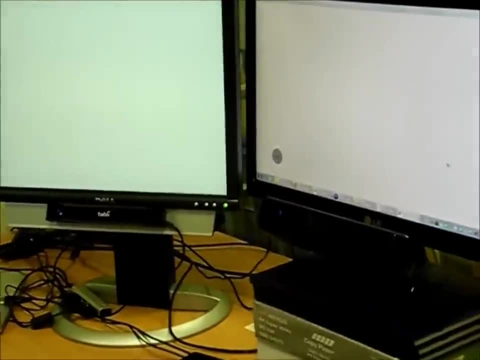 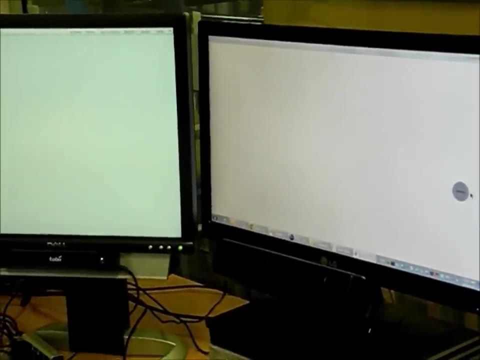 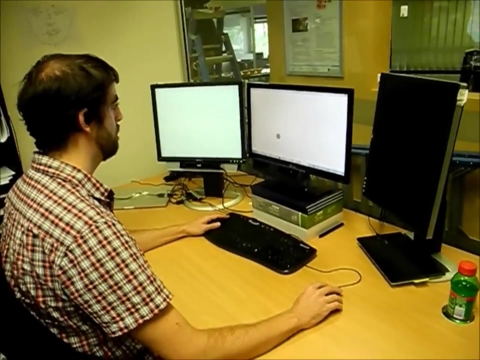 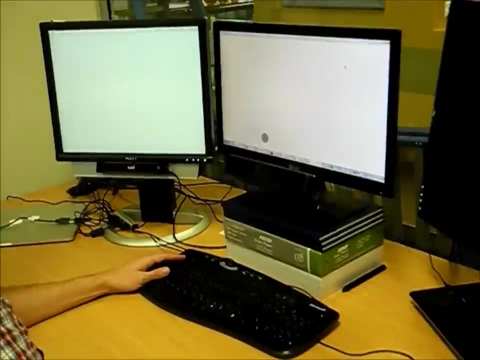